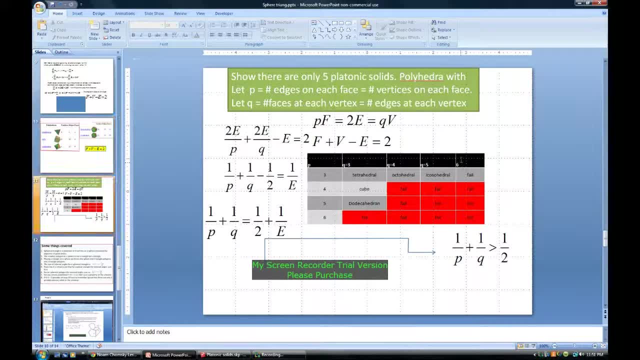 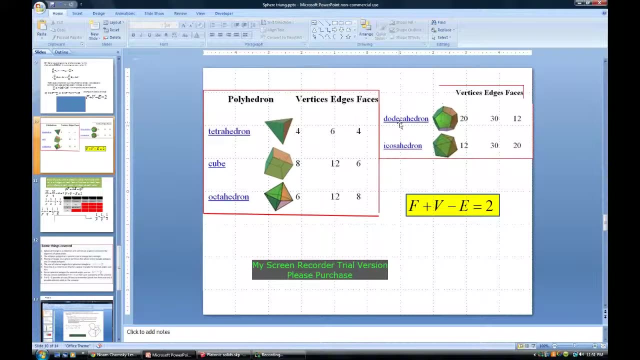 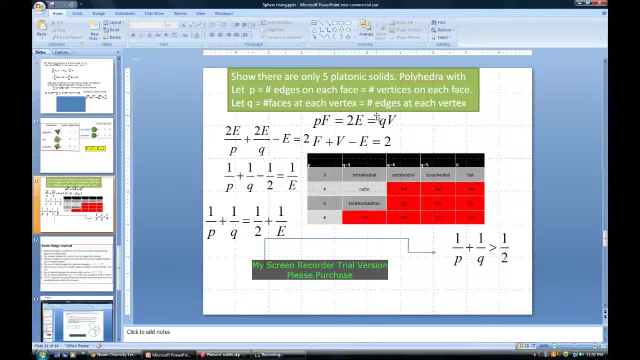 And I kind of want to show the proof using this logic: Let P equal the number of edges on each face, which is equal to the number of vertices on each face. So, And let Q equal the number of faces that come together at each vertex or the number of edges at each vertex. 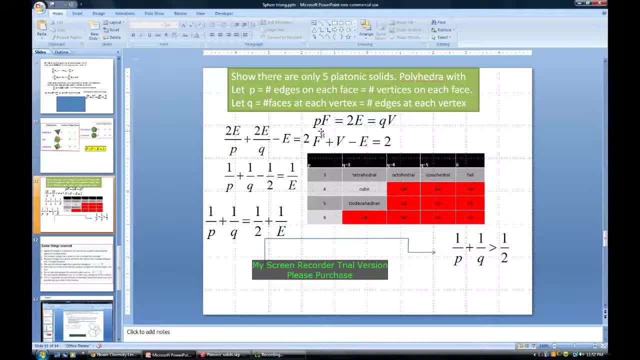 Now it's a fact that the number P- the number of edges on each face- times the number of faces is twice the number of edges, Because each edge is shared by two different faces. So you essentially go around to all the faces and count them all up and you'll be counting each edge twice. 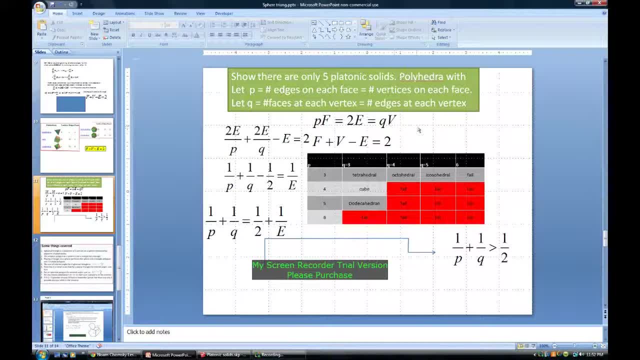 And the same thing holds for the vertices Two. Each edge is connected by two vertices. So if you count the edges at each face for every vertex, you'll be counting each edge twice, And so Q- the number of edges at each vertex, or meeting at each vertex, times the number of vertices, is twice the number of edges. 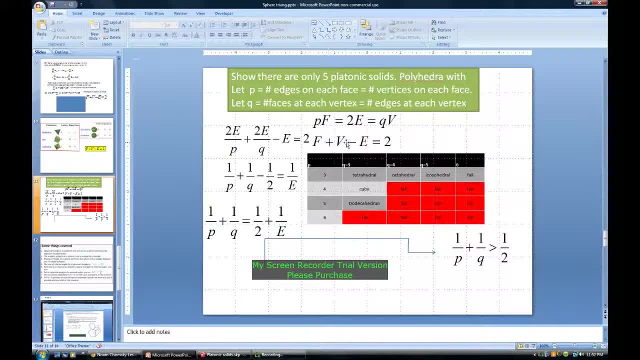 Then you can write this equation: F plus V minus E equals two over again As In terms of only E, because you can set F equal to two E over P and you can set V equal to two E over Q. So then you just get: instead of F plus V minus E equals two, you get two E over P plus two E over Q minus E equals two. 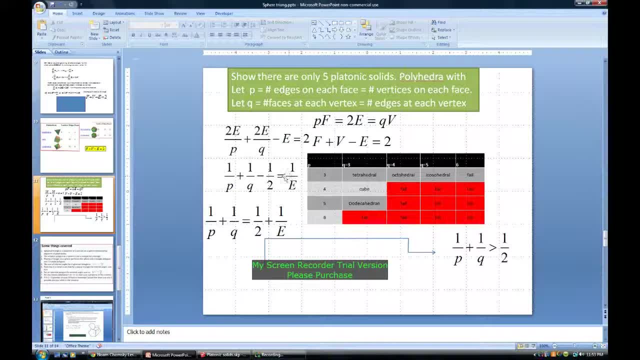 Always, always, always. And you can divide out the two E and you get one over P plus one over Q. minus one half equals one over E Or one over Q plus one over P or one over P plus one over Q equals one half plus one over E. 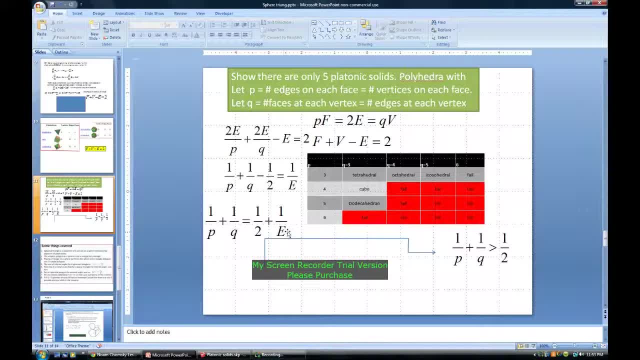 One over E is always a positive number, because the number of edges is always positive, So it must also therefore be true that one over P plus one over Q is greater than one half, And this works for any case where you have the same number of edges on each face. 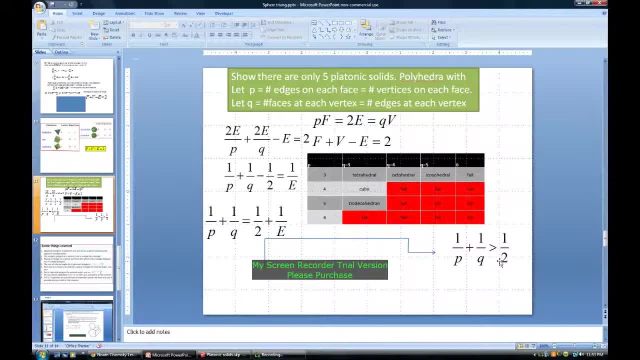 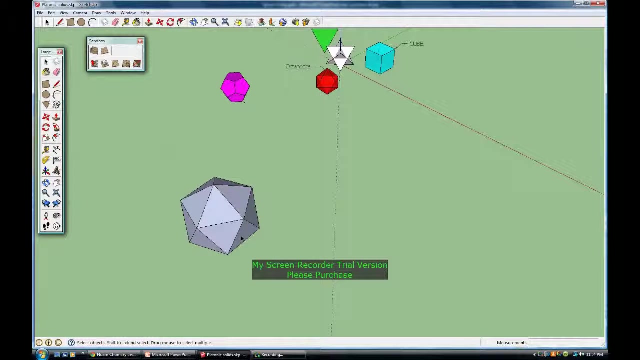 and the same number of faces And the same number of faces coming to each vertex and the same number of edges coming to each vertex. Now, because every face and every edge are the same, or all the faces are identical. So you could take one of these figures here, platonic, solid, and stretch it out. 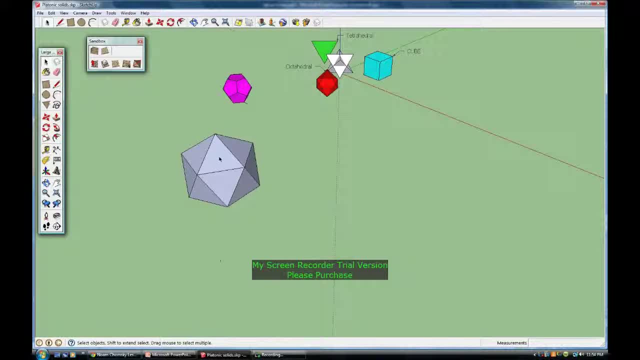 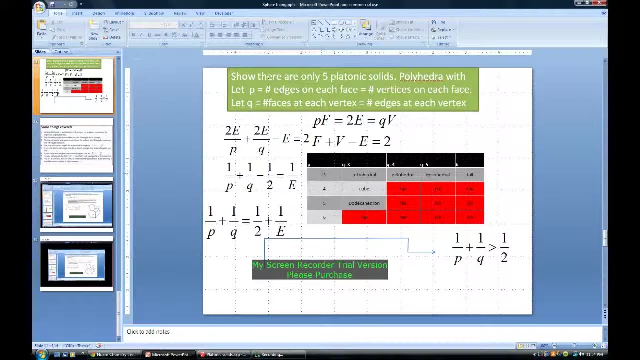 and then some of the faces would become longer than the other ones, and so forth. They would no longer be all identical. But since you can't do that and still have a platonic solid, then the relationship is preserved, And so you can make this table up for when the inequality is satisfied. 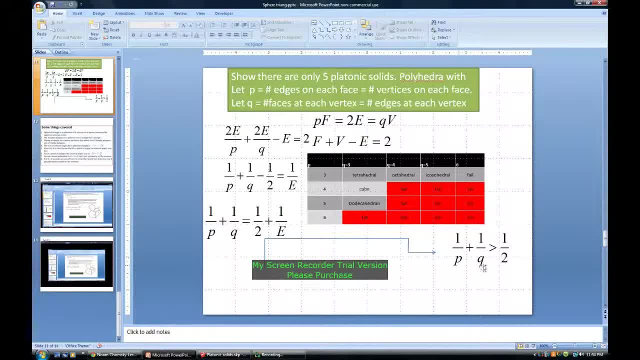 Obviously it can't be satisfied, for like say, P equals 100 and Q equals 100, because that's just two one hundredths, That's far less than one half. So P and Q must be more or less small numbers, and three is the smallest number. 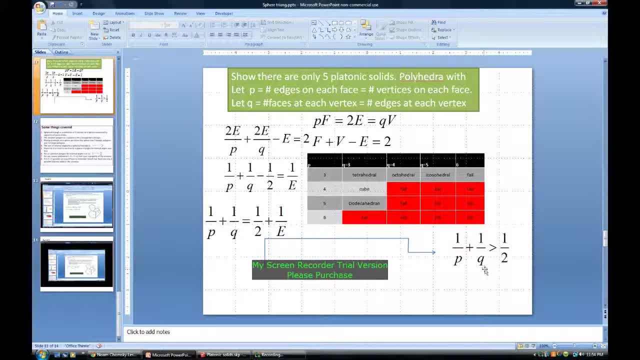 because the faces are in Euclidean space, They have to be. the smallest is a triangle with three faces, three edges on each face. So you can look through here It obviously works for P equals three and Q equals three. the tetrahedral. 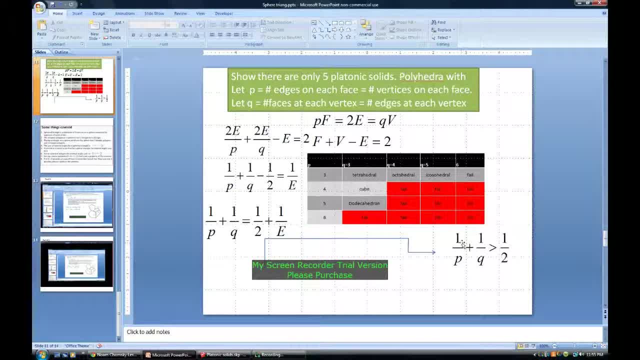 because one third plus one third is two thirds bigger than one half. all the way up until you get like a case where three and five are working together and you have one third plus one fifth. If you put that in terms of fifteenths, that's five fifteenths plus three fifteenths. 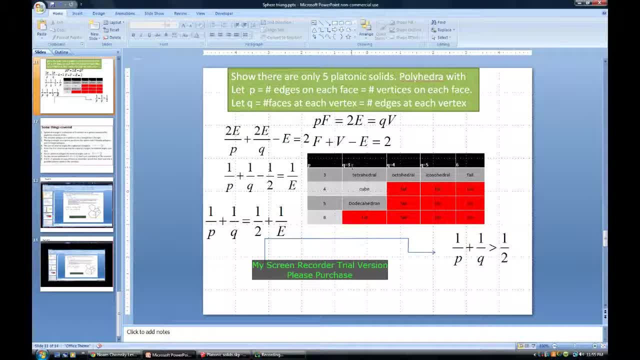 eight, fifteenths, still bigger than one half. But it fails once you get to three and six, because that would just be if you had one third, one over three plus one over six. that would turn out to be nine over eighteen, which is exactly one half. 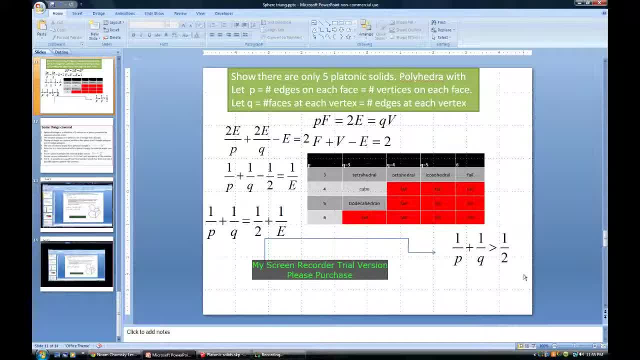 So that's basically the algebraic proof for why there can only be five platonic solids. I just want to throw that in there as one last final application for the Euler characteristic for polyhedra in three-dimensional space.